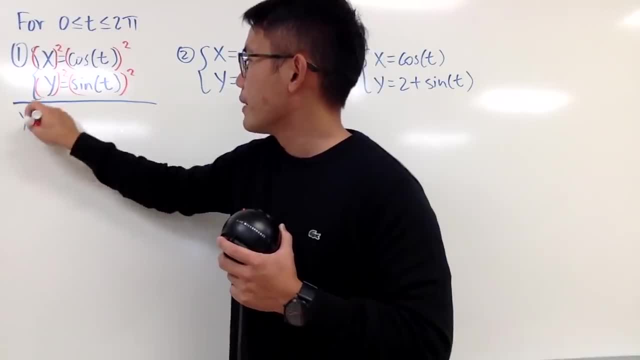 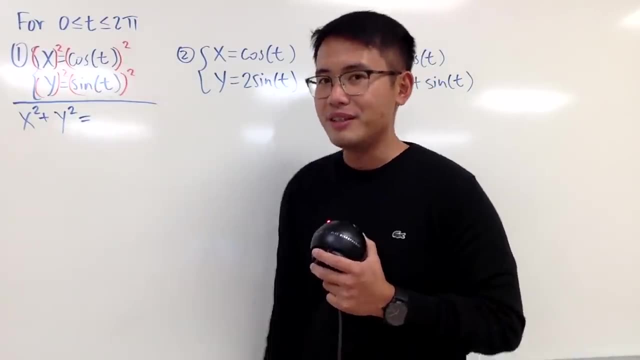 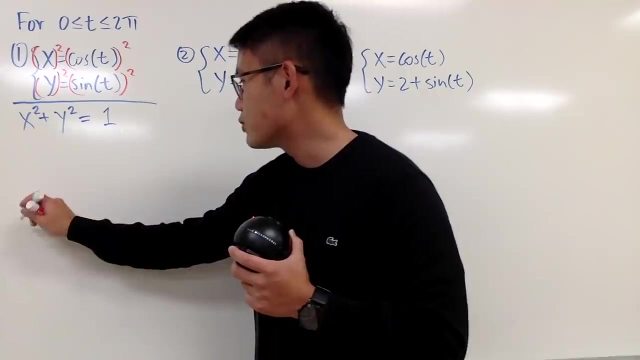 left-hand side, you see that you will have x squared plus y squared, and here you have cosine squared t plus sine squared t, and that's equal to 1.. So, as you can see, this is of course the unit circle. now, And let me just demonstrate by drawing a picture, right? 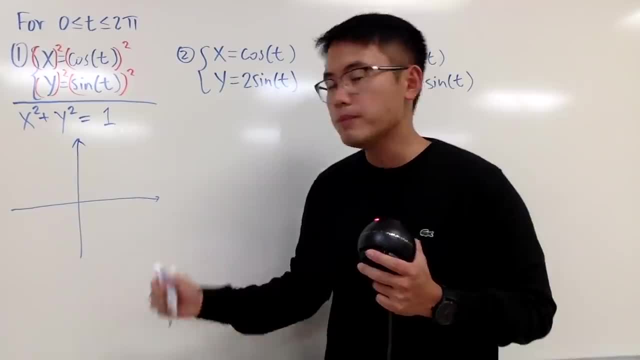 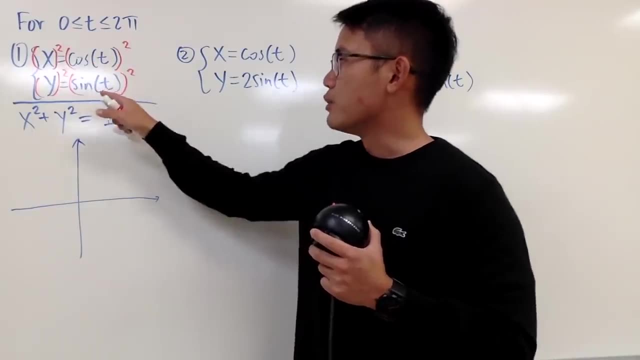 here, And you can do it with a table, It's all up to you. When t is 0,, you start at 1,0, because cosine 0 is 1 and sine 0 is 0. So you start right here. This is 1,0, and this. 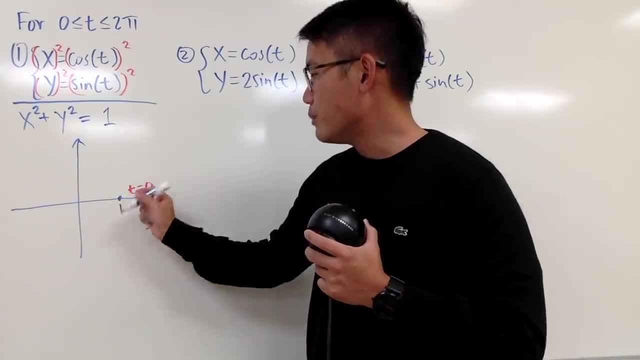 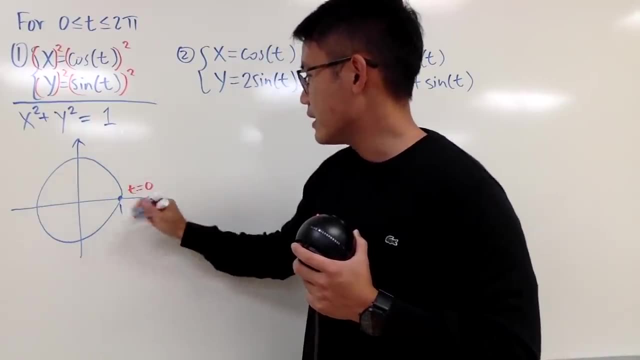 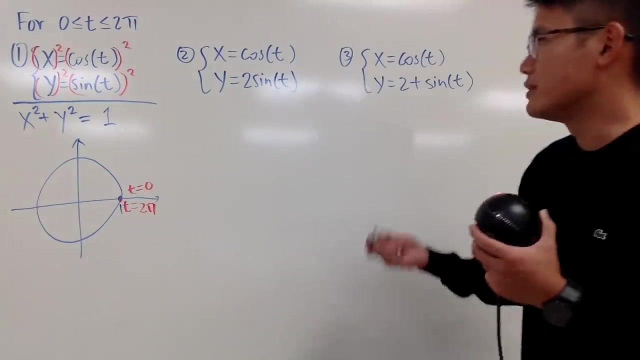 is when t equals 0. You pretty much travel counterclockwise, So you go like this, like that, and then you end up with when t is 2 pi. So this is just a pretty standard unit circle. Now let's. 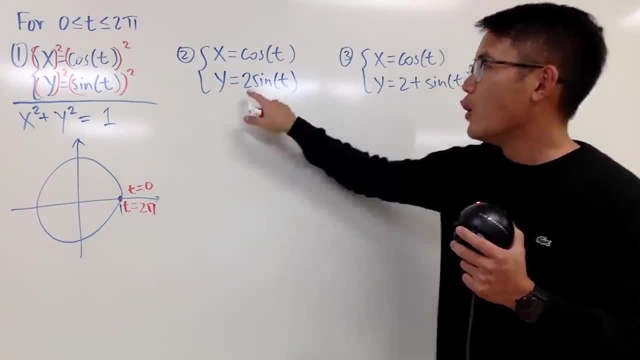 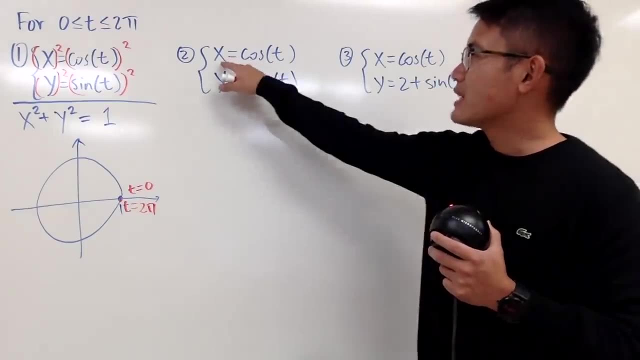 talk about this right here, And the only difference between this and that is we have a 2 in front of the sine t. Well, well, what do you guys think? This time the x-value is still cosine, but the y-value, you know, it's still cosine. So, it's still cosine, but the y-value you. 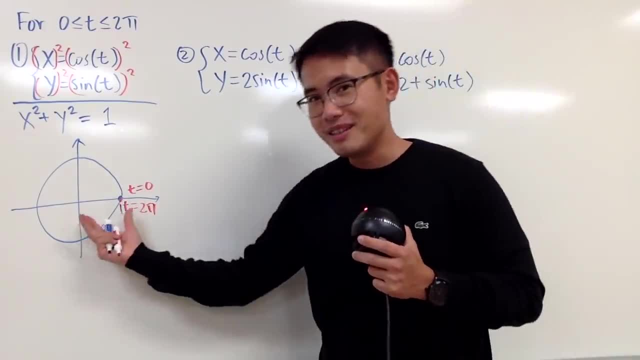 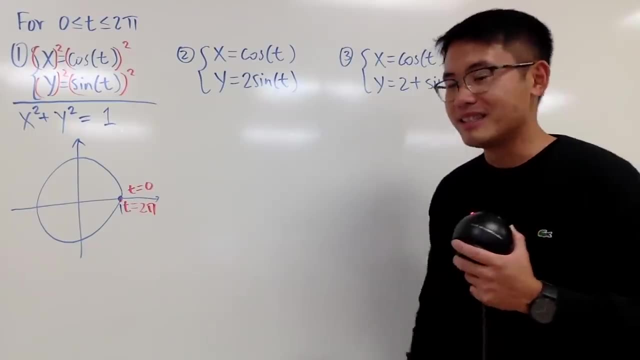 know it got multiplied by 2.. It's still going to be this kind of thing. However, you pretty much stretch the y-values right by 2 like this, So in fact, you get an ellipse like a vertical situation like that, And, of course, if you want to change this to the Cartesian, 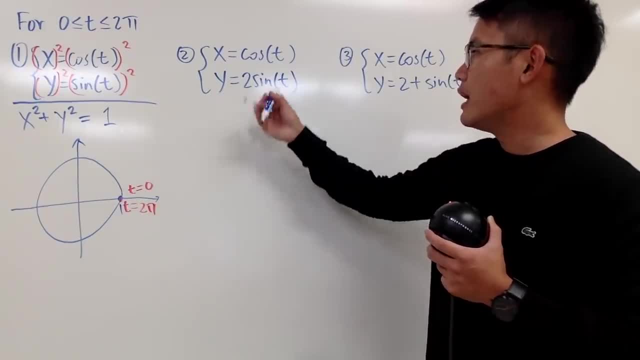 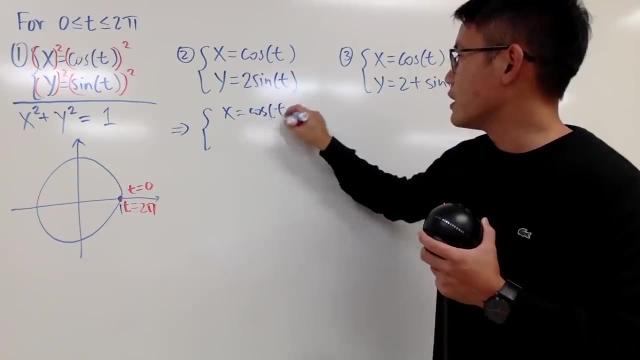 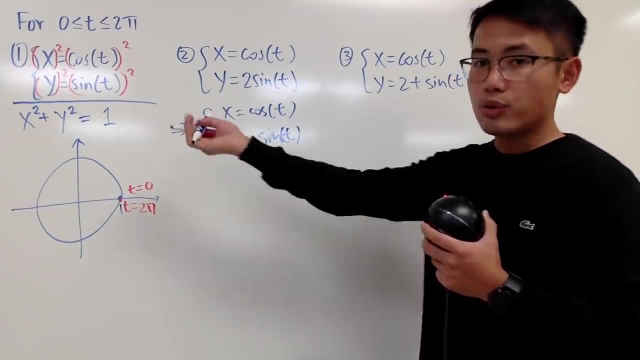 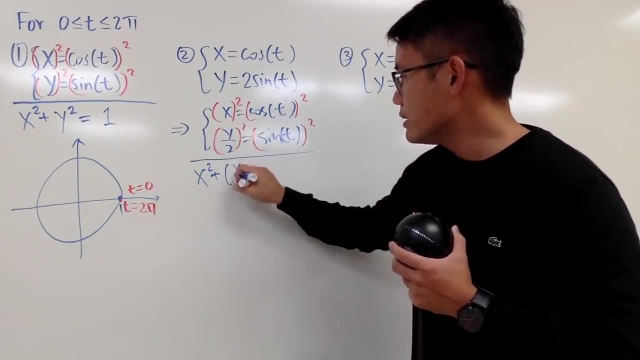 equation, you will have to divide both sides by 2, and you pretty much will see that this is the same as saying x is cosine of t and then y over 2 is equal to sine of t. So you can do that again. When you add these two equations here, you have x squared plus parentheses. 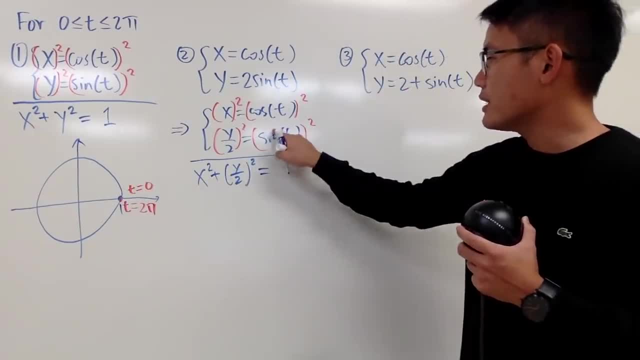 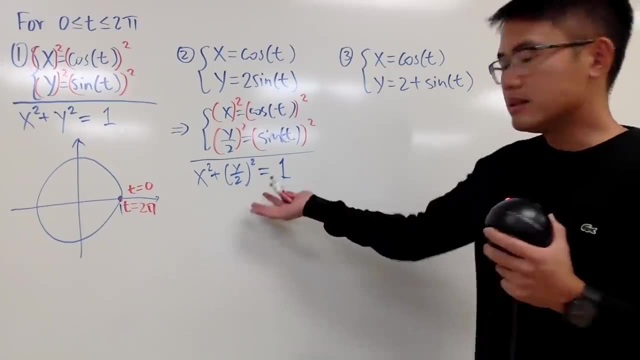 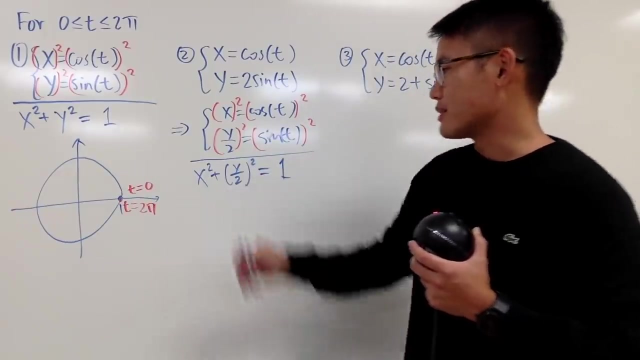 y over 2 squared and this is equal to sine squared plus cosine squared is just 1, as the 1 over there, And this is pretty much the equation for ellipse, and you can see the y-intercepts are 2 and negative 2, and then you'll know when x is 0.. So anyway, 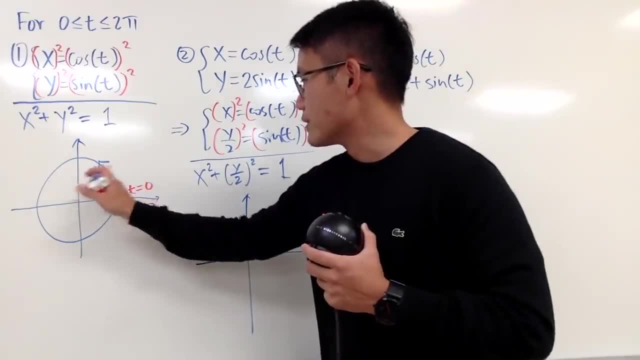 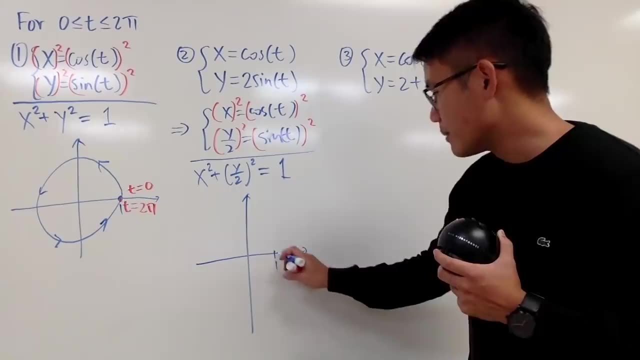 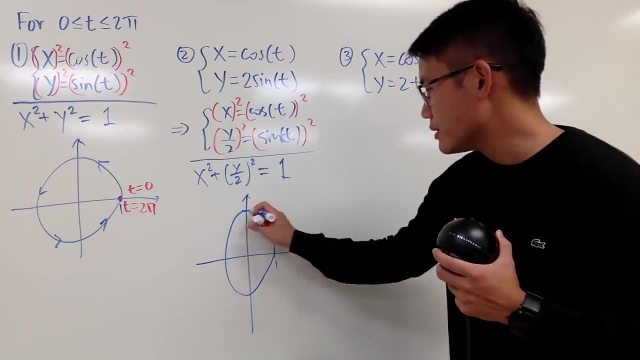 enough said, I'll show you guys the picture. Oh, by the way, I should draw the arrows like this when you are talking about parametric equations. This right here is similar. You start at 1, 0.. You go like this up to 2,, though, and then you go down to negative 2.. So this: 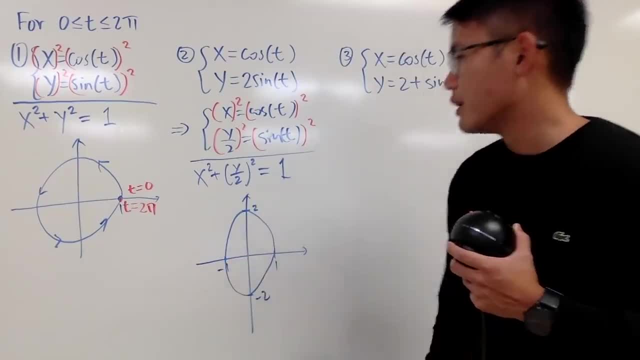 is 2,, then this is negative 2, and, of course, this is negative 1.. And over here it was all 1s. Anyway, this is pretty much it. So you can draw the arrows like that and this. 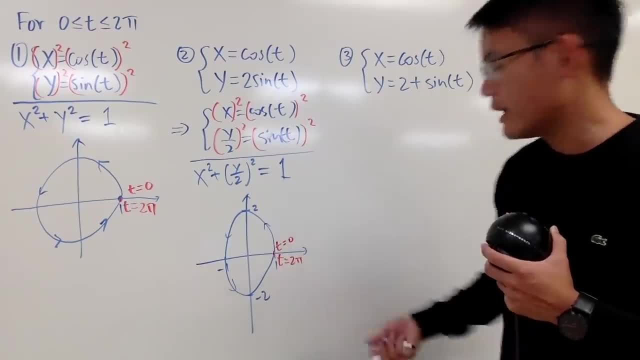 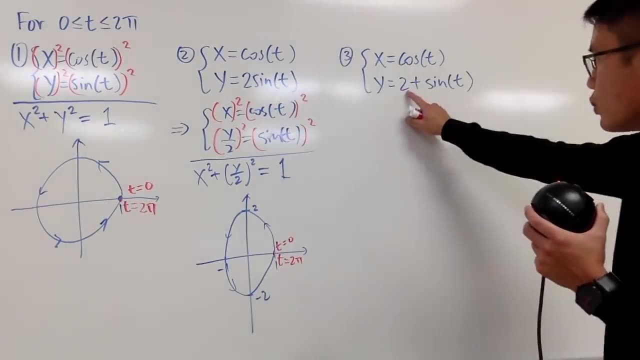 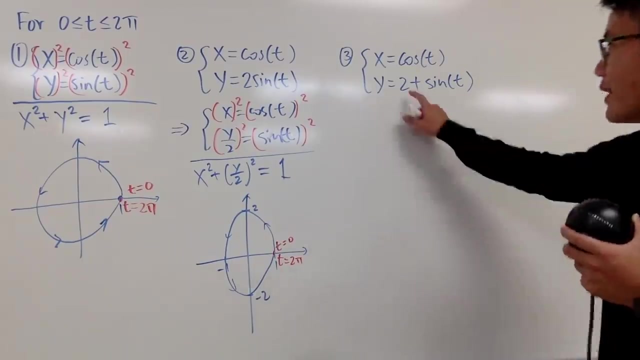 is when t equals 0 and t equals 0.. t equals 2. pi like that, and we're done. Lastly, instead of multiplying the sine by 2, we are adding 2 right here with the sine t. So what do we get? Well, you're adding. 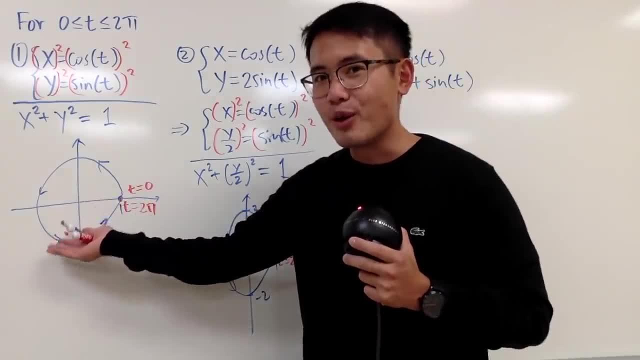 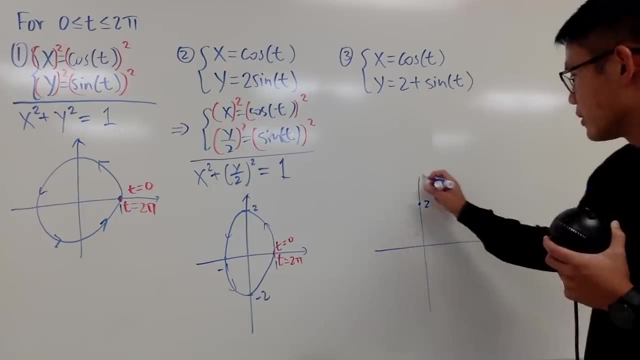 2 to the y values. You just pretty much bring the circle up twice. So that's pretty much. you can just do the circle with you guys. first Do the unit circle like this, and this is going to be negative 1.. Anyway, that's pretty much the idea. and yeah, this is 1, this is. 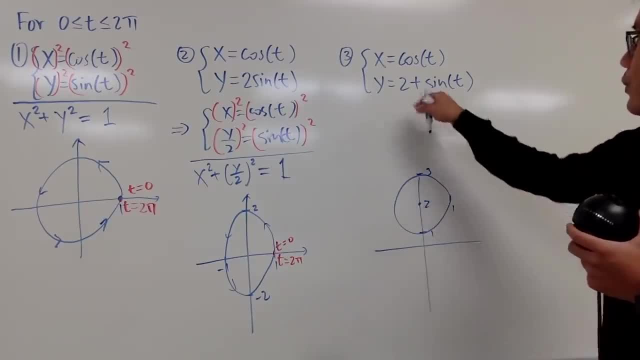 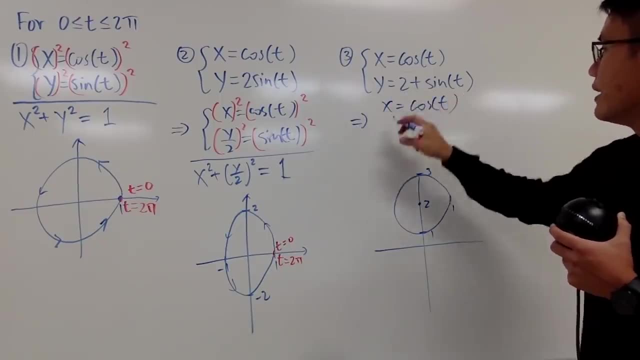 going to be 3, and this is going to be negative 1, of course. Well, to see that you can just minus 2 on both sides. So you see, this is the same as x equals cosine of t, and then 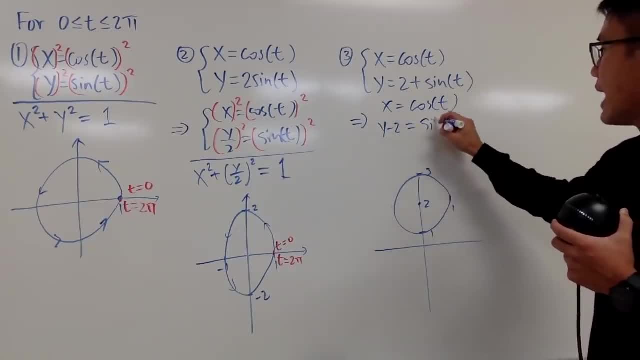 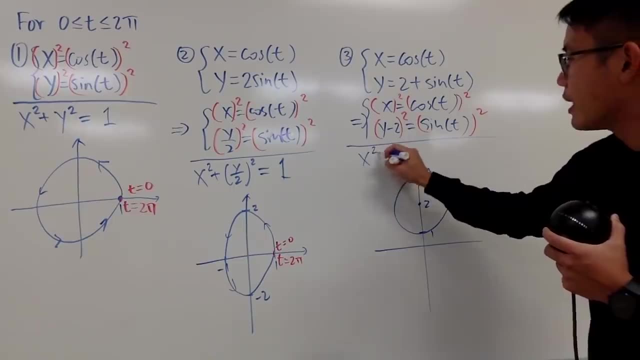 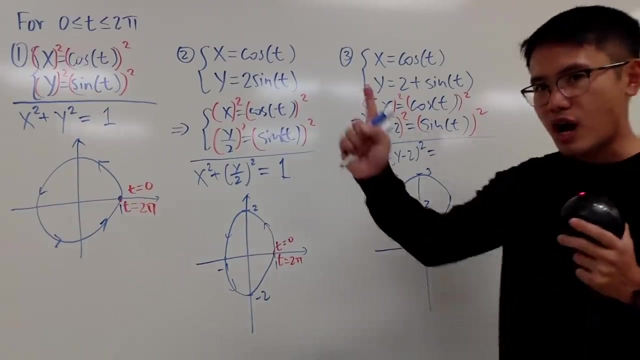 the second equation: y minus 2 equals sine of t. And then you do that again and then add the equations Here, you get x squared plus parentheses, y minus 2, and then, squared cosine, squared plus sine squared, we get 1.. So this is the circle with radius 1, centered. 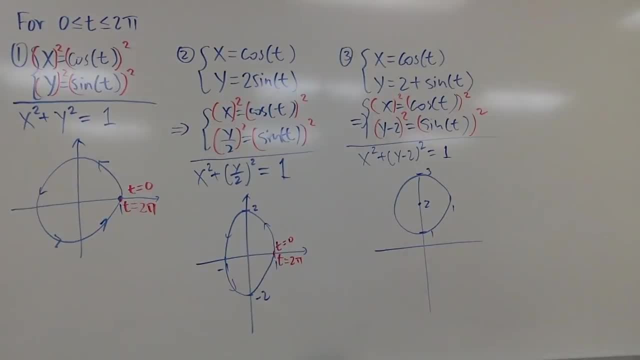 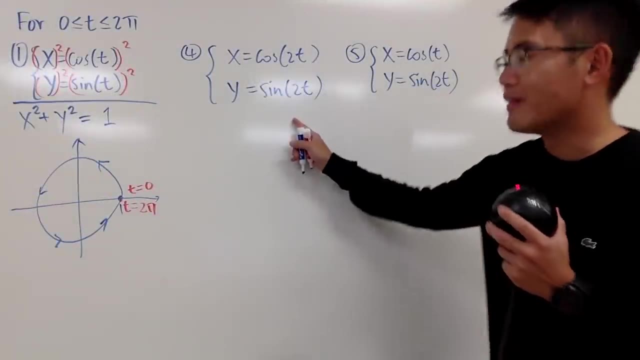 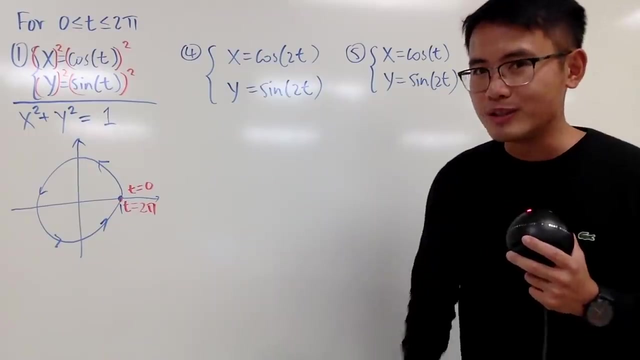 at 0, positive 2.. Okay, continue, Here. we have this one right here We have: x is equal to cosine of 2t and y is equal to sine of 2t. Yes, we just multiply the t's by 2.. So what does this do now? Well, 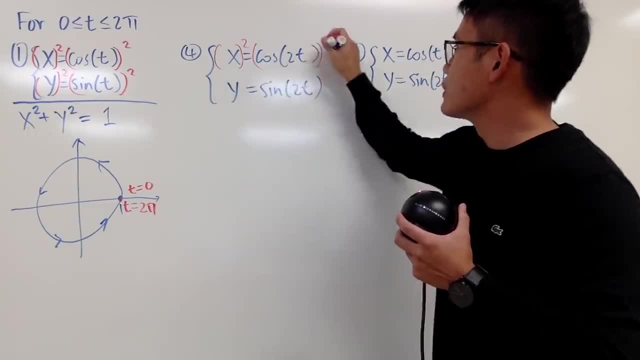 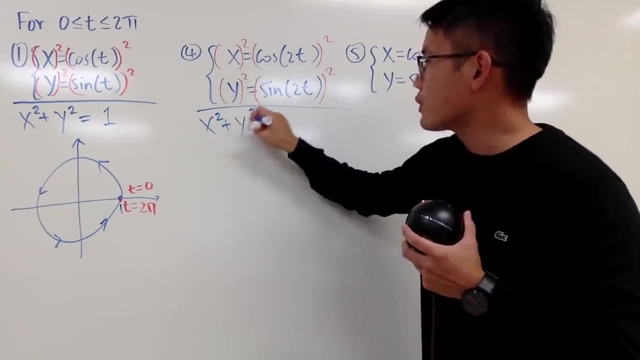 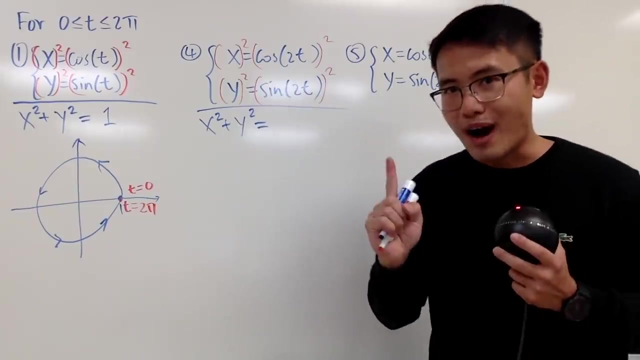 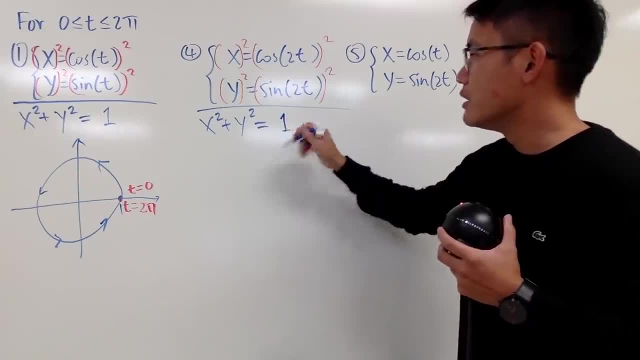 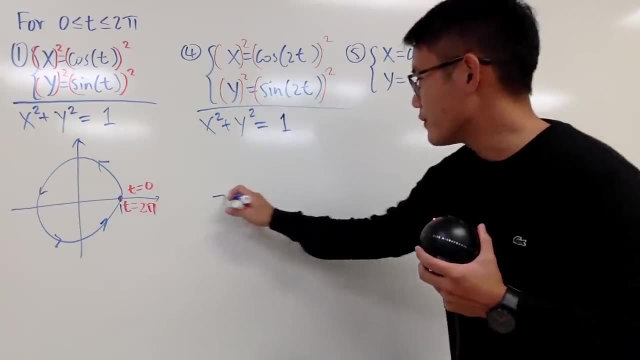 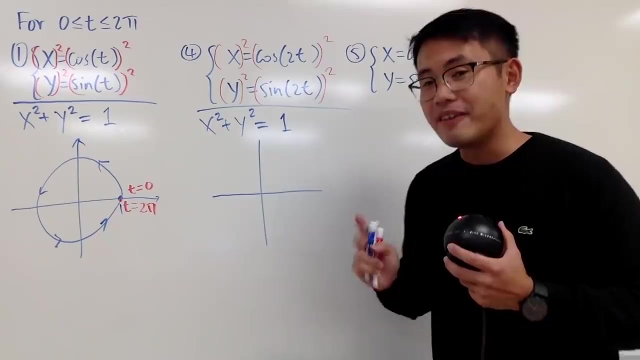 the angles are the same, So we still end up with the unit circle. So is there any difference between this and that though? Yes, of course, But let me draw a picture for you guys right here. So we still get the unit circle By the moment that you multiply the t by 2, in fact you. 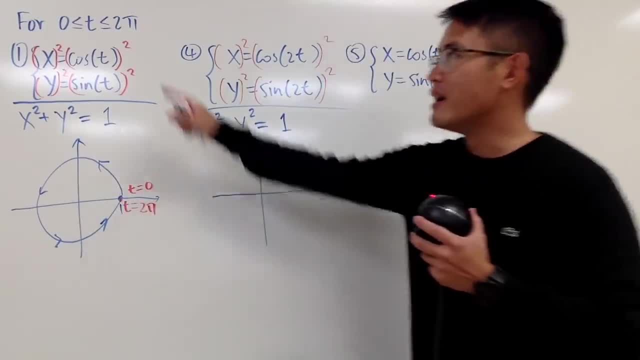 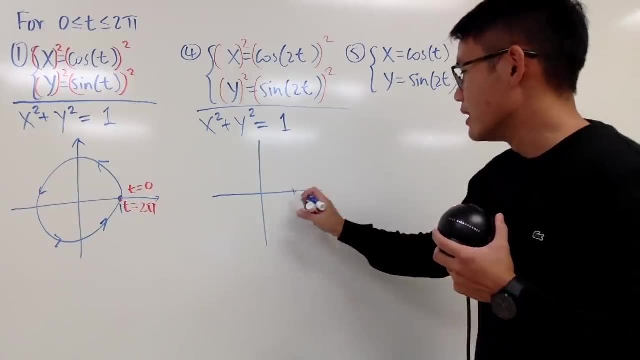 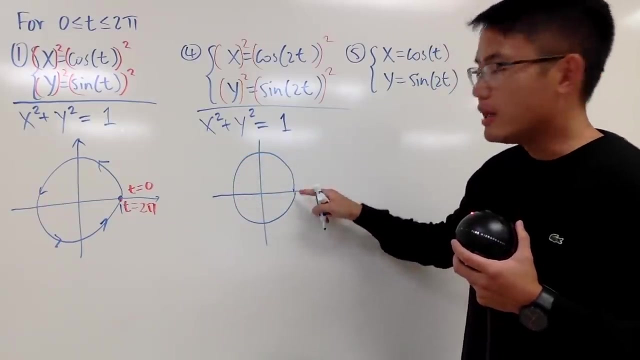 are going to run around the circle twice in the same time period, because you are pretty much going twice as fast as the original. So the picture is going to be like this: You start at 1 comma 0, and you will go counterclockwise like this one time and you will see this: 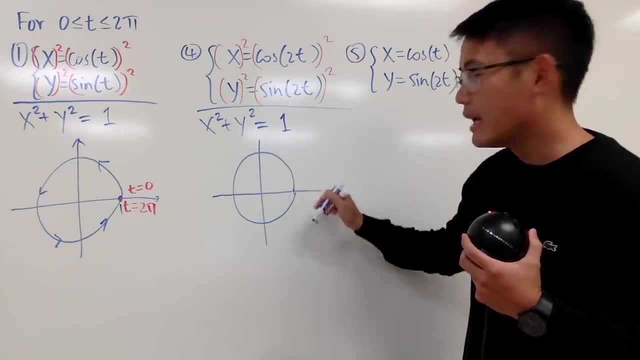 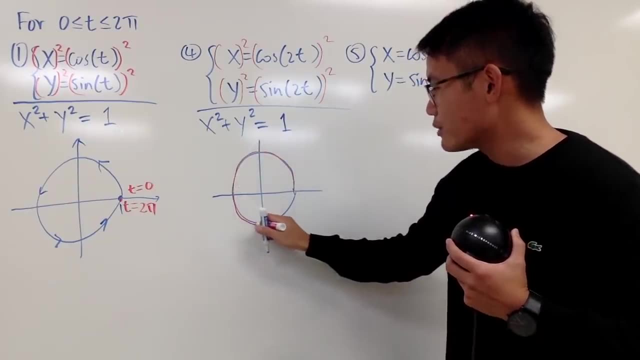 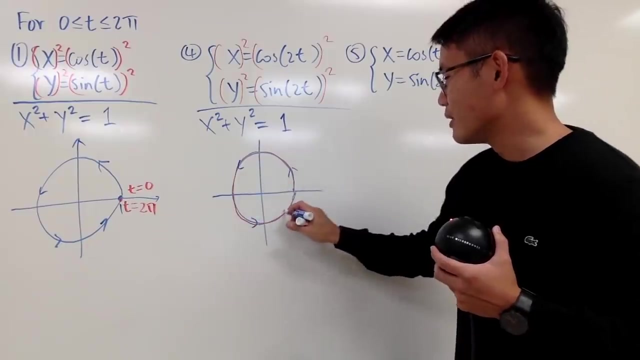 is when t is equal to 0, and then t is equal to pi, and then you will continue because you have more time, because you are running twice as fast, So you can actually do another loop again. So you actually pretty much do this twice. That's it, So let me just draw. 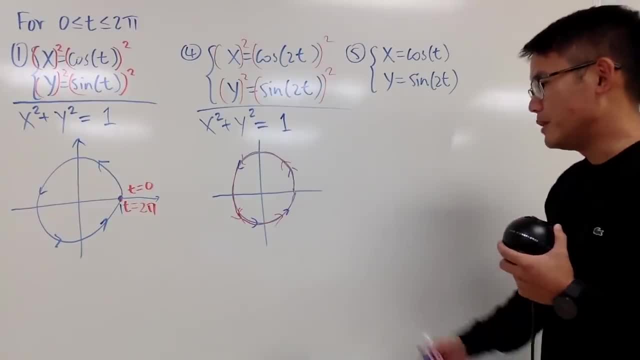 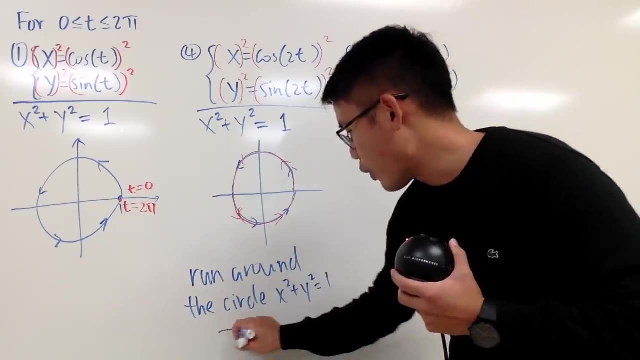 the arrows right here. So you should draw the arrows. and maybe you say we're just going to run around the circle. I will just say the circle is x squared plus y squared, which equals 1, twice. And you can imagine if you multiply this by 7 and 7, yes, you'll run. around the circle. Now, what you're talking about is the ate squared plus y squared equals 1 twice X squared equals y squared. So I used an evolutionень like that And you can imagine if you multiply this by 7, and 7, yes, 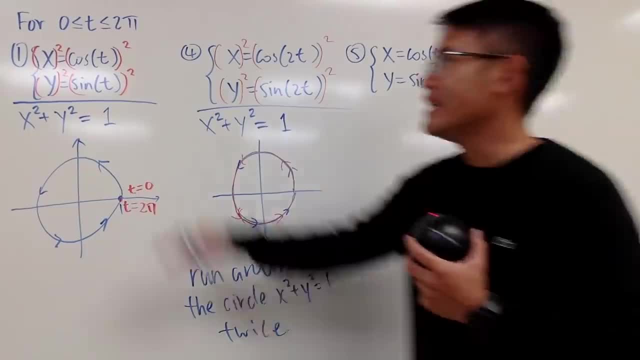 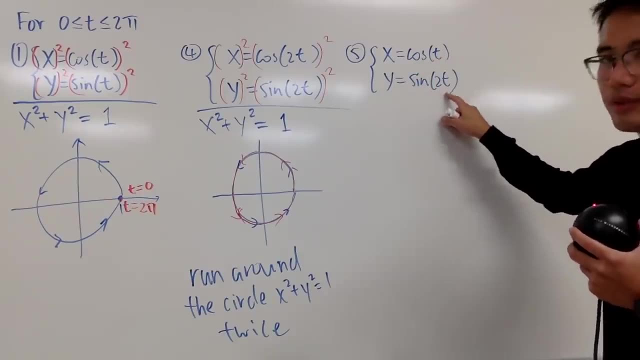 and 7, yes, you run around the circle 7 times in the same time period, Alright, last example: Here we have: x is equal to cosine of t and y is equal to sine of 2t. Unfortunately, the angles are different. 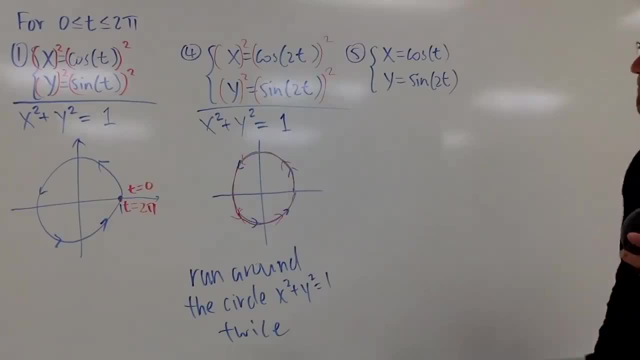 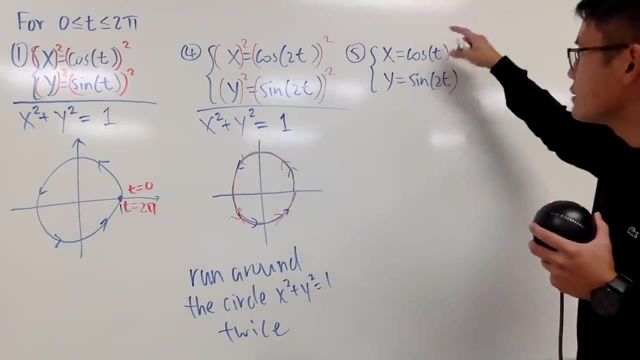 And let me tell you, we don't end up with a circle right here. Hmm, what can we do? I actually cannot square both sides like that, because when the angles are different, then cosine squared t plus sine squared of 2t. 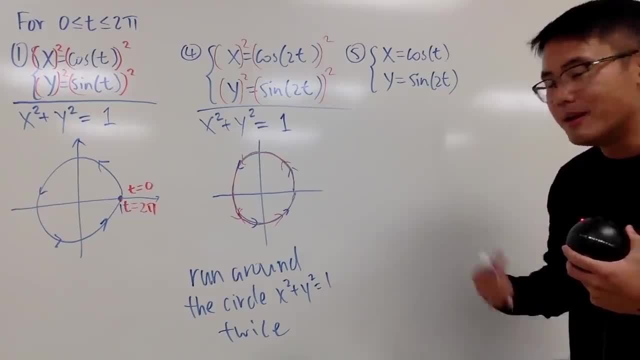 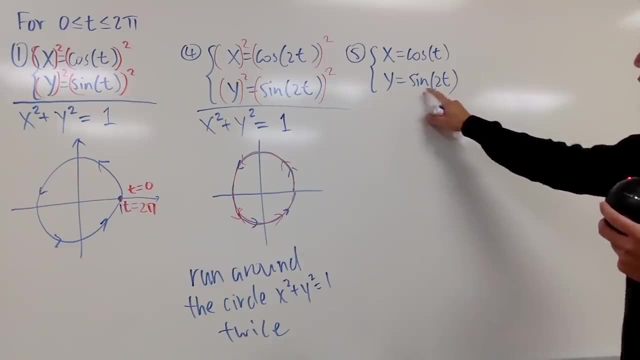 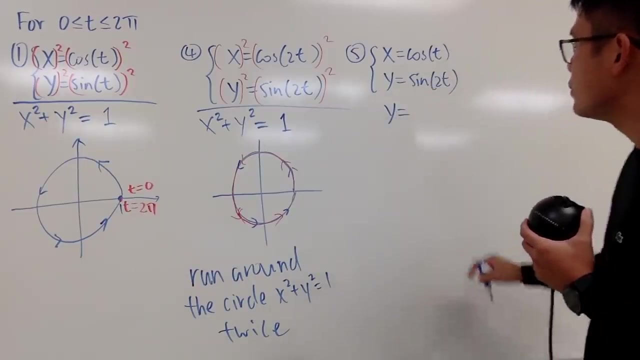 I cannot do anything unless I do more tricks. identity, And this is what we can do. I will do the identity right here, because I notice I have y equals sine of 2t. I can use the double angle identity for sine, So I will write down. we know y is actually equal to. 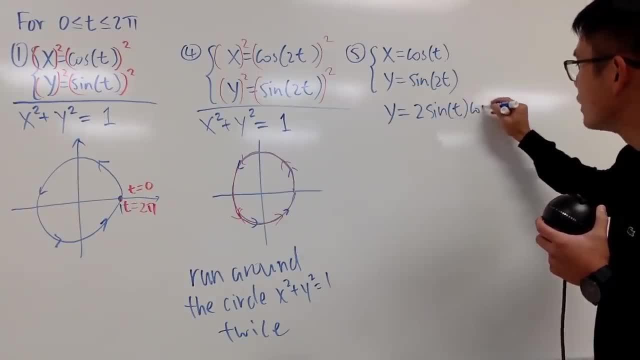 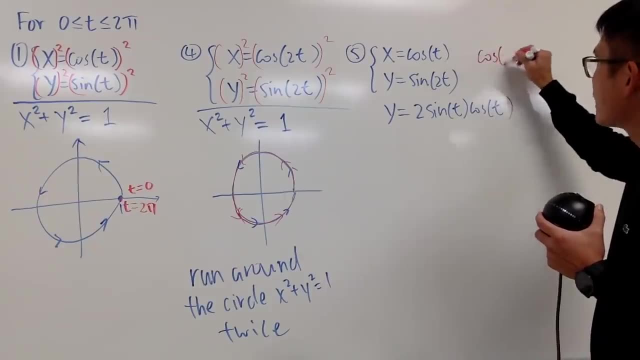 this is the same as saying 2 sine of t times cosine of t. And now you see, cosine of t is just x. And let me write it down right here: Cosine of t is equal to x. That's good. 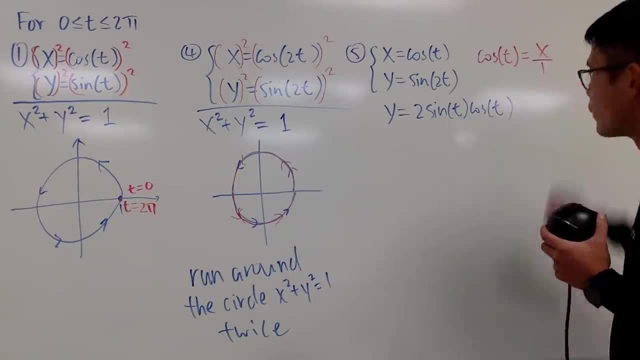 But I can make it better. I will make it x over 1. Because I need to use this information to figure out what sine of t is. And how can we do that? Yes, we draw triangles Right triangle specifically. so let's do it right here. 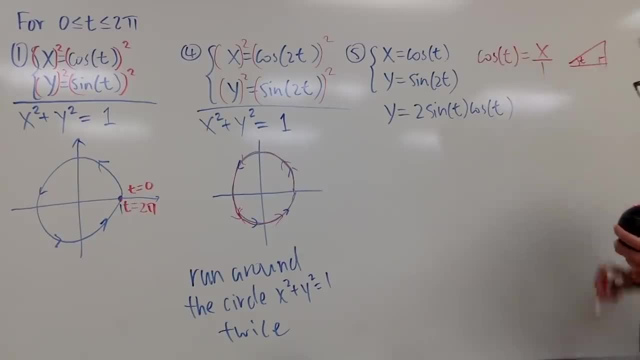 This is my right angle And this is my angle t. And because we have cosines, so this is the adjacent on the top, which is this right here. And because we have cosines, so this is the adjacent on the top, which is this right here. 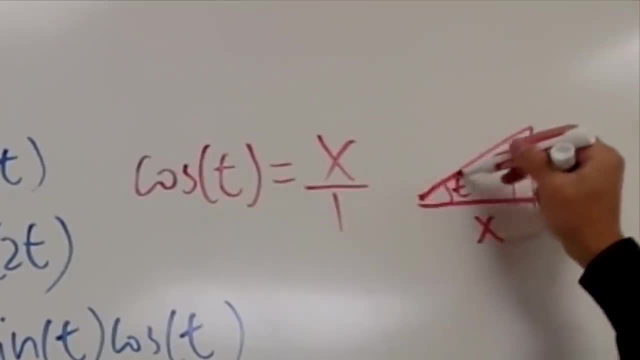 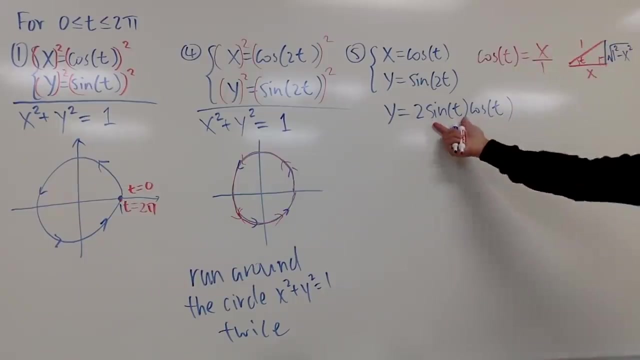 That's x, And the one will be the hypotenuse which is right here, which is 1.. And you have to write the opposite, which is the square root of 1 square minus x square. like that, And based on that picture, we can figure out what sine of t is. 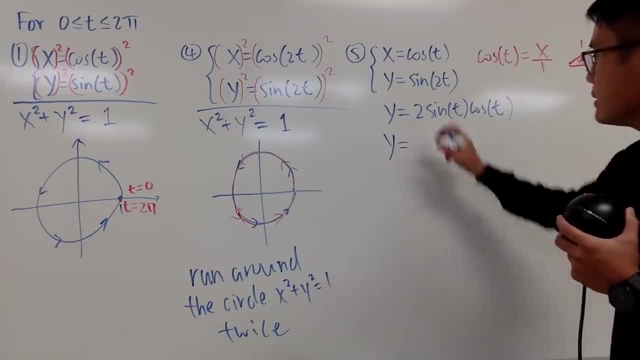 And let's go ahead and do that. We have y equals 2.. And for sine of t, this is just the opposite over the hypotenuse, which is square root of 1 minus x squared. And then for cosine of t, it's just x, pretty much. 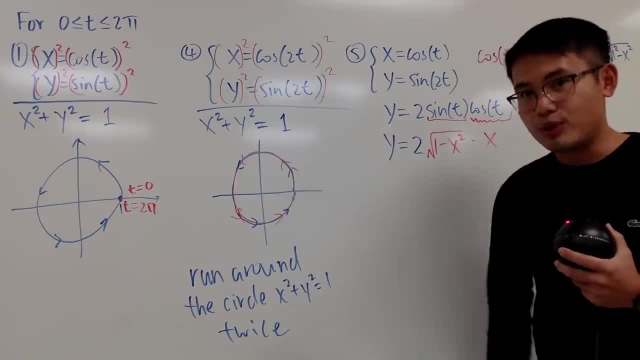 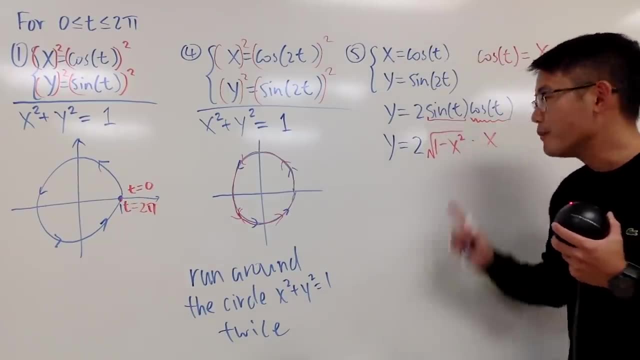 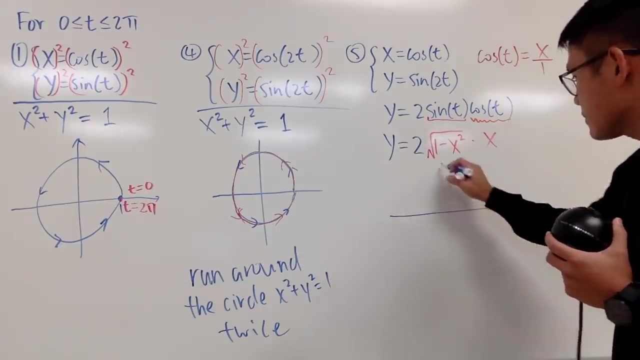 So this right here, you multiply by x, So that's pretty much it. That's how we can get this parametric equation into the Cartesian form. Unfortunately, though, if you just grab this right here because of the square root, let me tell you guys, your graph is going to look like this only: 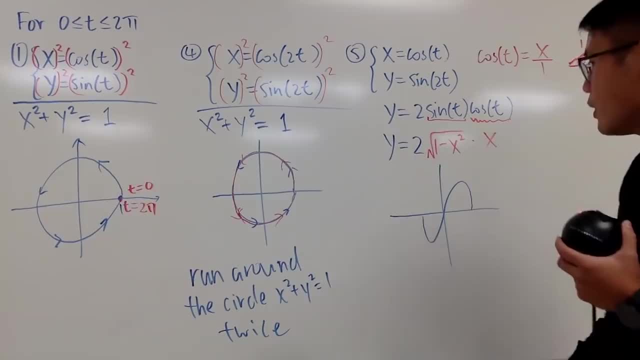 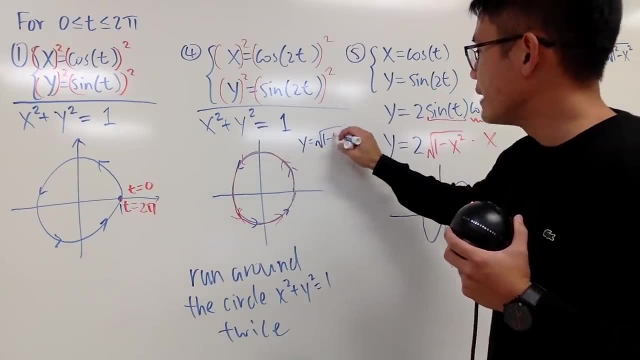 Why? Because you have the square root. Well. well, you can imagine: if you solve for y right here, you will end up with y equals square root of 1 minus x squared, And this, right here, will only give you the top. 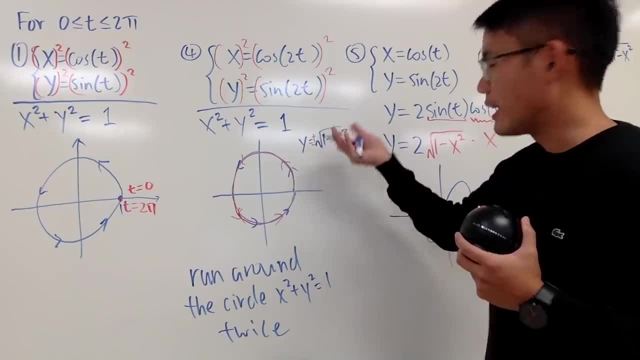 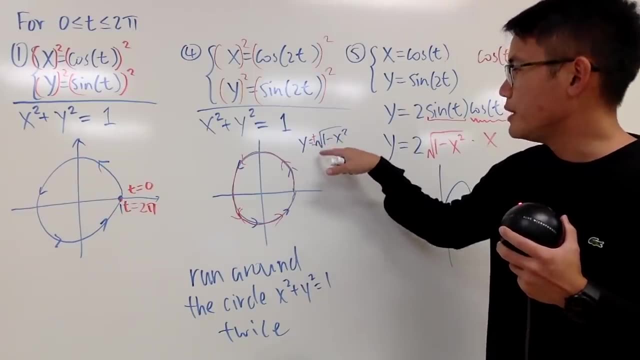 In order for you to do the bottom, you have to actually have the plus minus right. Well, you see, this is troublesome. when you isolate the y, You have to talk about two pieces: the positive and also the negative. This was more complete. 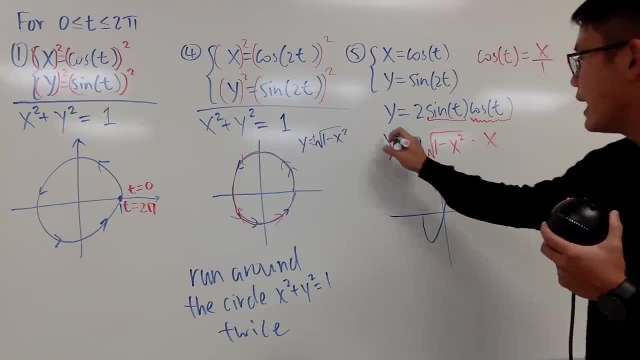 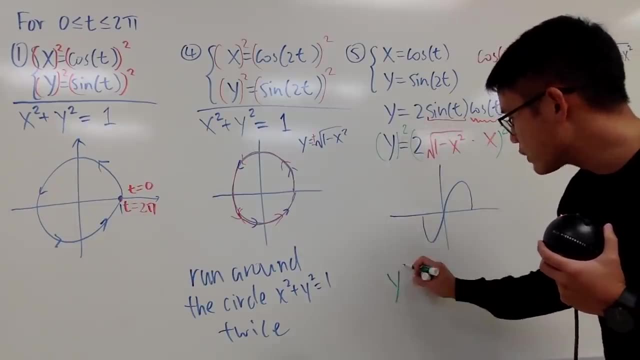 So the way to take out this problem is this: is that okay, let's just go ahead and square both sides here And I'll write down the answer here. On the left-hand side, I will end up with y squared.